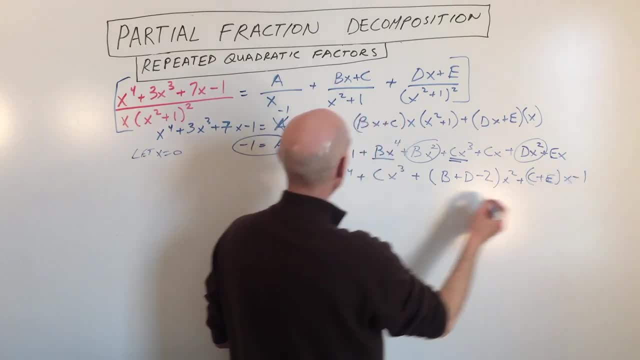 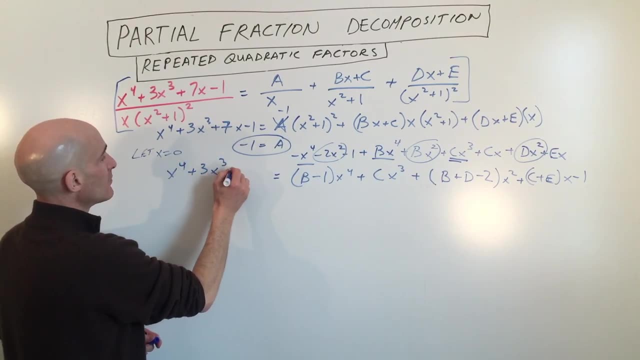 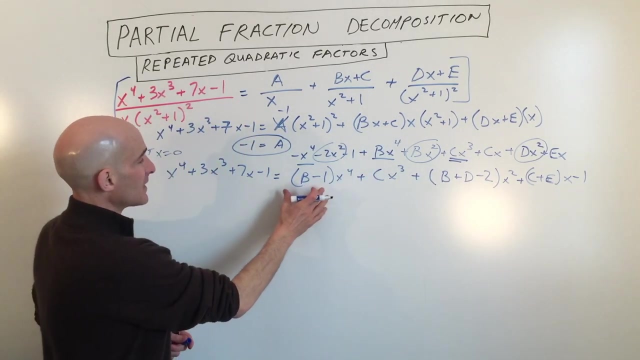 Okay, so we can say this is minus 1 equals x to the 4th plus 3x cubed plus 7x minus 1. So we're going to solve this equation, and we're going to do that by setting b minus 1, the coefficient in front of the x to the 4th term, equal to this coefficient, which is 1. So we have b minus 1 equals 1. Okay, so you can see b is going to equal 2. 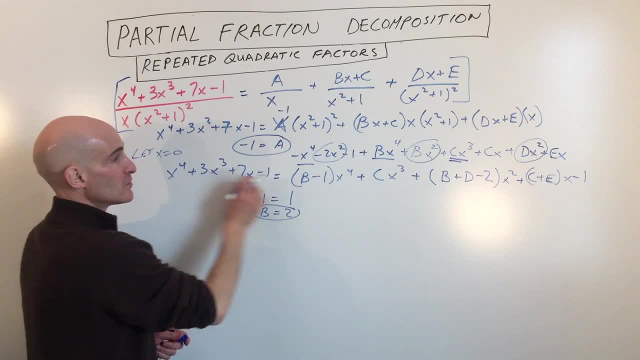 Now we're going to set the x cubed is equal to x cubed. So you can see that c equals 3. Okay, c equals 3. 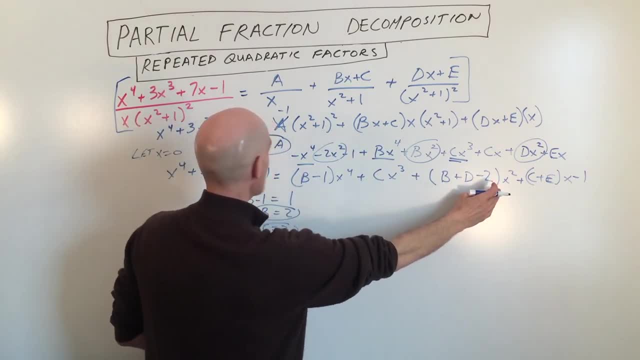 And we're going to set the coefficients in front of the x squared terms, b plus d minus 2. 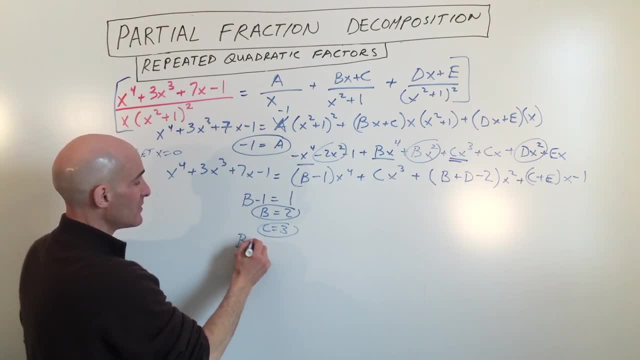 And you can see there's not an x squared term here, so that's going to be b plus d minus 2 equals 0. 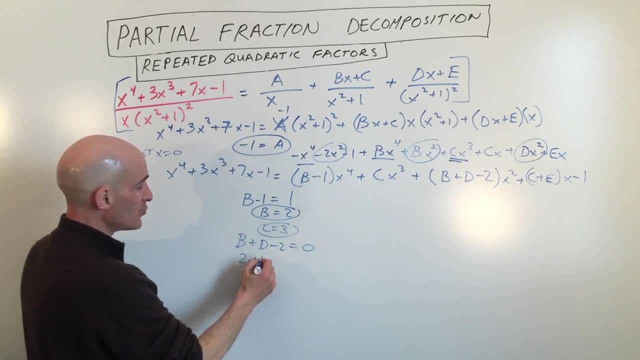 Okay, and because we know that b is 2, that's going to be 2 plus d minus 2 equals 0. Those cancel, so you can see that d equals 0. 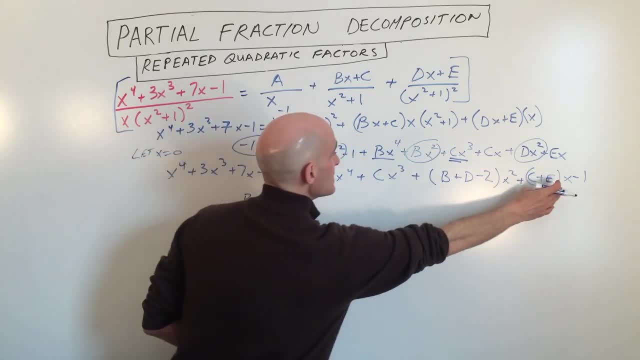 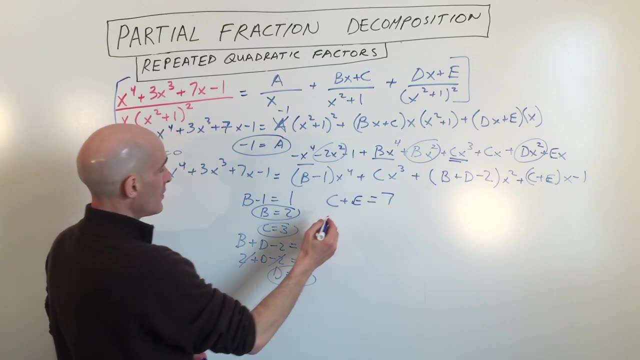 And then the last one, let's see, we've got c plus e, which is the coefficient in front of the x. That's c plus e equals 7. Okay, and we know c is 3, so that's 3 plus e equals 7. So we know that e equals 4. 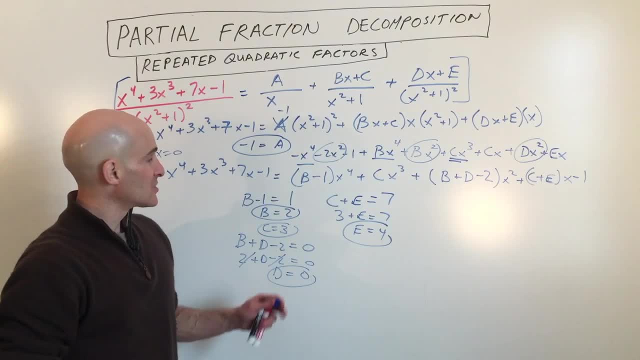 And negative 1, of course, equals negative 1. Okay.